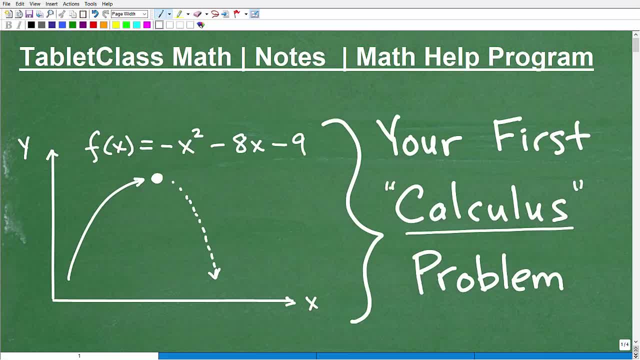 And calculus has kind of a reputation of being advanced and difficult, and in fact it is. But the concepts and principles are actually pretty, you know, understandable for anybody and are very beautiful. So calculus is such a powerful mathematics. So the whole point of this video is to kind of introduce you to some of the power of calculus. 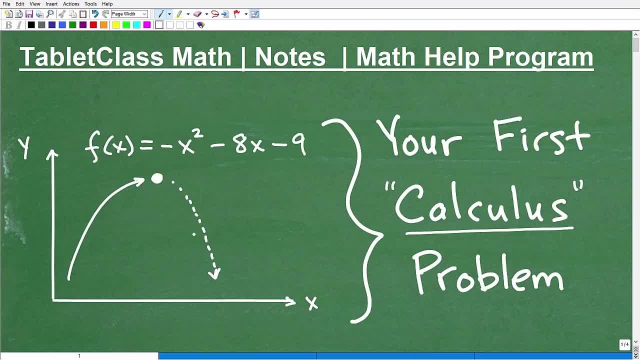 Okay, and we're going to be doing something here. It's going to be kind of a little basic, interesting problem, And if you've never done calculus before, stick around, because this could definitely be your first calculus problem And we'll kind of solve it together. 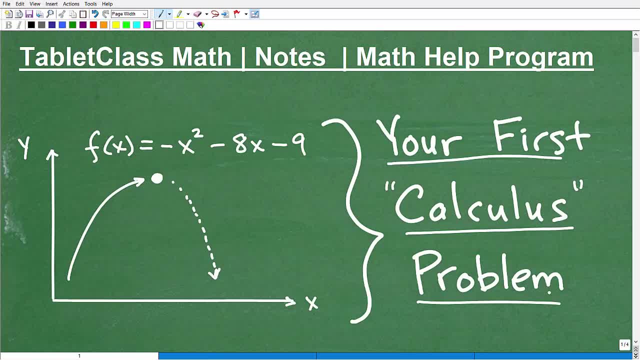 But I will say in full disclosure that I'm going to be doing some algebra- Not much, Okay, some basic algebra in this problem. So if you're not familiar with algebra, still stick around. Okay, you'll learn something. But if you know some algebra, you'll kind of relate to some of the things I'm going to be talking about here in a second. 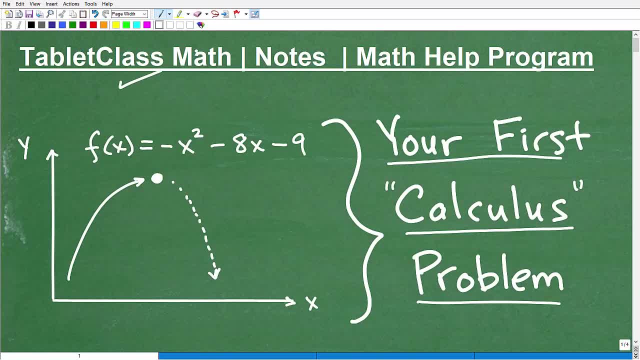 But first I'm going to quickly introduce myself. My name is John. I'm the founder of Tablet Class Math. I'm also a middle and high school math teacher And over many years I've constructed what I like to believe is one of the most robust, comprehensive online video-based math help programs there is. 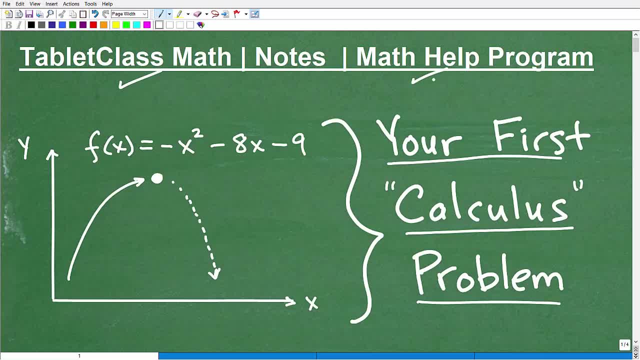 Now, of course, I'll let you be the judge of that if you want to check it out. But you can find a link to my math help program in the description of this video. But whether you need to take a full, comprehensive math course, I can help you. 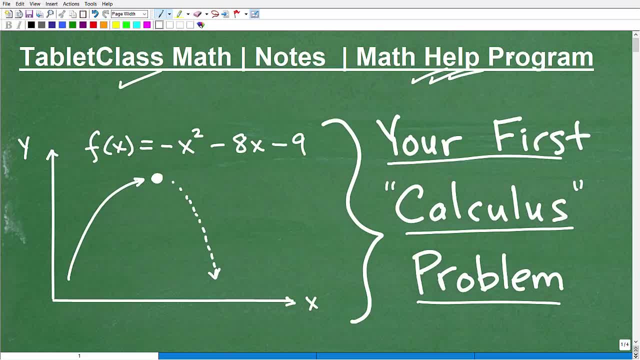 Or you need assistance in a course you might be taking right now. I can help you. All my courses have full, comprehensive lessons And I teach you how to solve the most common type of problems you're going to be facing at the middle high school level or even more advanced levels. 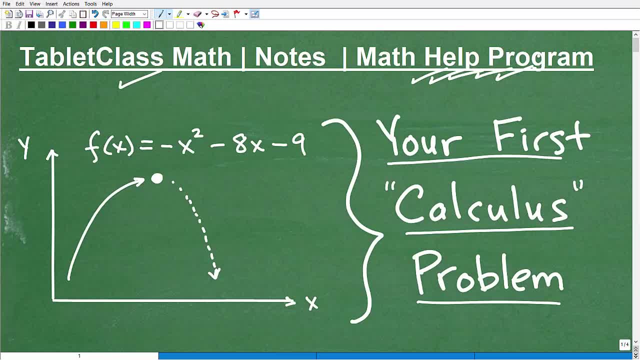 Okay, I literally solve thousands of problems And I think that's where my program is very unique. Okay, not many programs really have that much video content, But again, if you're interested, you can follow the link in the description below. 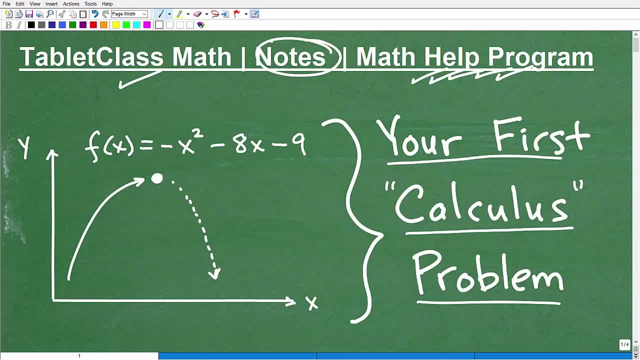 Okay, now let's talk about math notes. If you are a math student, you may or may not be, but if you are a math student, you need to have outstanding math notes. Okay, after decades of teaching math, one thing is apparent to me. 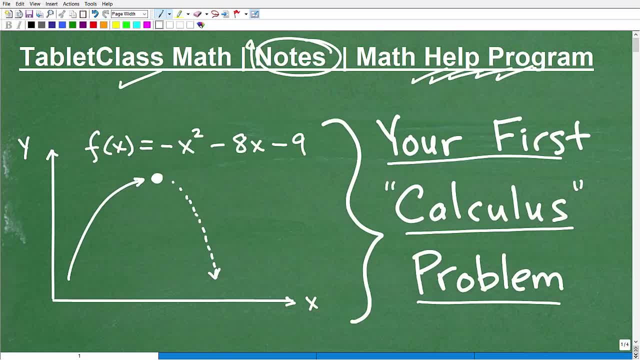 Those students with the best math notes almost always have the best math grade, And the reverse is true. Okay, those students with no math notes, sloppy, disorganized math notes, And that was me way back in the day. I had to learn how to take math notes. 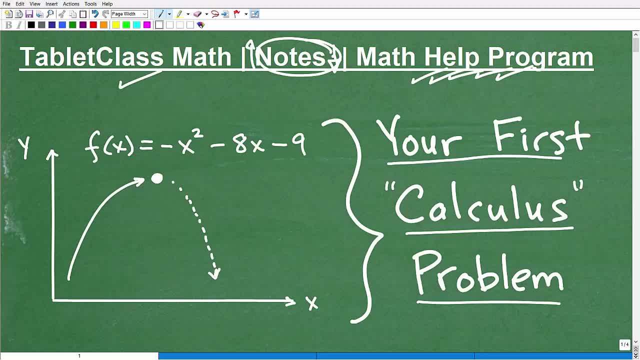 And that's maybe your situation. Okay. so if your notes are not that great, don't get down on yourself too much. Just recognize that you have to start improving, Okay, but in the meantime you need something to study from. So I actually offer very comprehensive, detailed math notes. 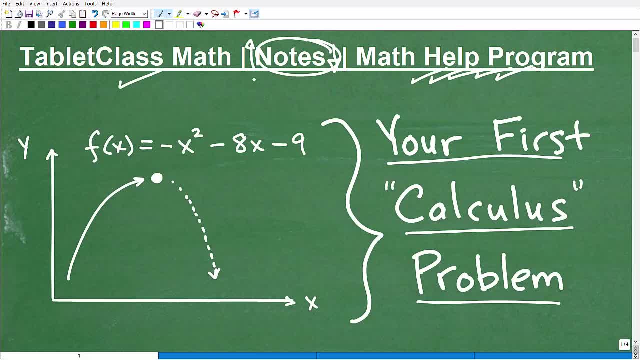 You can find a link to those in the description of this video as well. Those would include preoperatives Algebra- Algebra 1,, Geometry- Algebra 2, and Trigonometry. Okay, so let's get into this problem. And you might be saying: well, what is this problem? 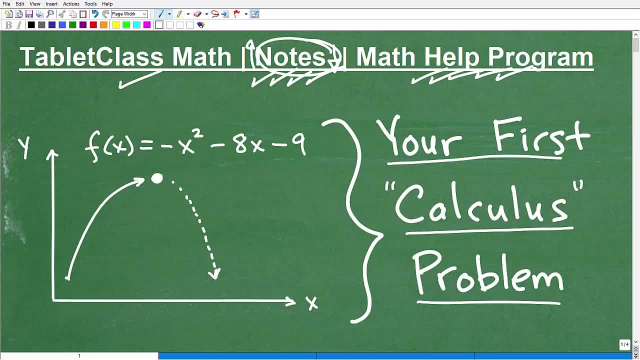 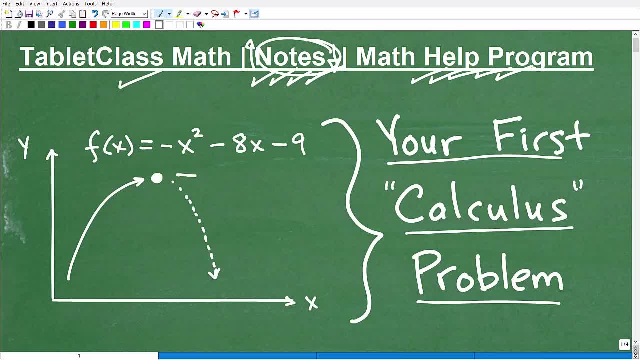 And now it's on its way back down. All right, so let's try to identify: at what point does this ball reach its maximum Maximum altitude? Okay, that's kind of the general idea here. Again, it's not going to be an exact. 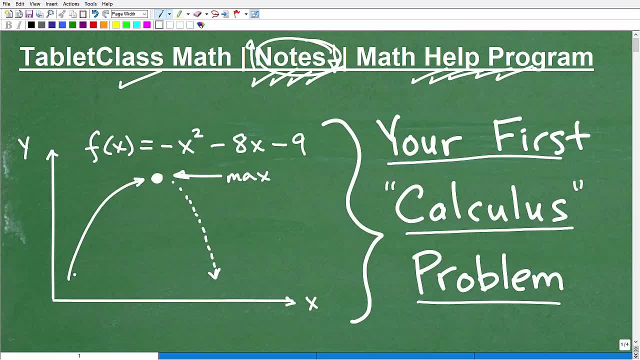 This would be like an example of physics problem. Okay, of course physics uses calculus. All the sciences use calculus as the mathematics, The more you know when you study them at a higher level. But we're going to basically find the maximum of a shape. 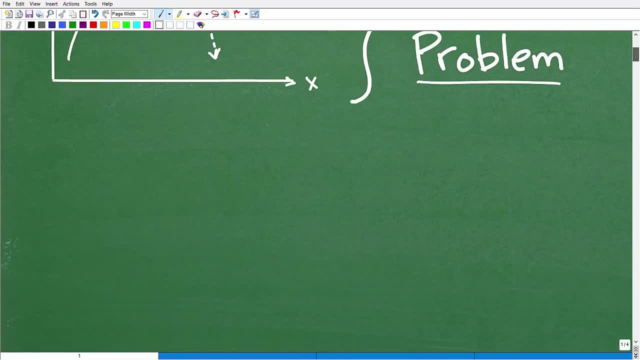 All right, and I'm going to do that in just one second, But let's kind of emphasize why this is so unique. Now, if you've taken algebra, you might recognize this, The shape here, as a parabola. Okay, it's a parabolic shape. 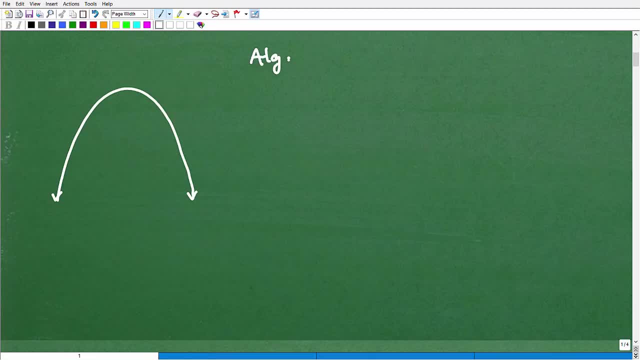 And we can just use some other algebraic techniques to find what we call the vertex. All right, which is? this point up here, Okay, which is the maximum, But I'm going to show you how we can use calculus to find this point as well. 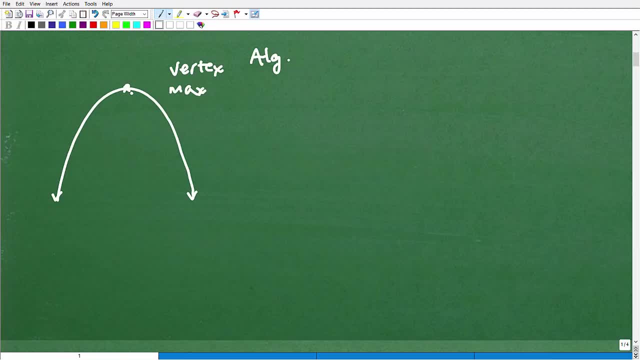 Because this is a nice illustration, basic illustration, of calculus. Now in calculus, when you learn calculus, okay, there's pretty much two big primary concepts that we learn. Okay, big picture topics. let's just say The first one is integration. 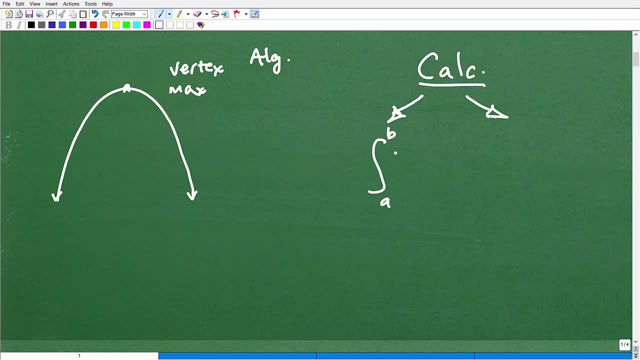 Okay, integration is a little symbol like this. You've probably seen this before. Looks kind of crazy, like so, And let's suppose this was on an XY chart right here. Integration is basically the way we can find area underneath a curve with something. 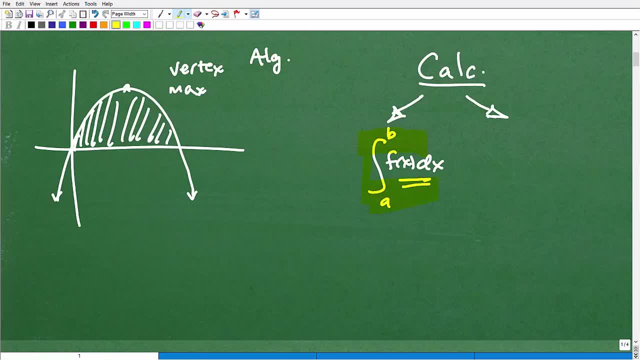 Okay, so very, very powerful. I've done a few videos on the basics of calculus. So we learned integration. Then we learned this other thing called the derivative. Okay, the derivative kind of looks like this symbol: DX, DY or Y prime. 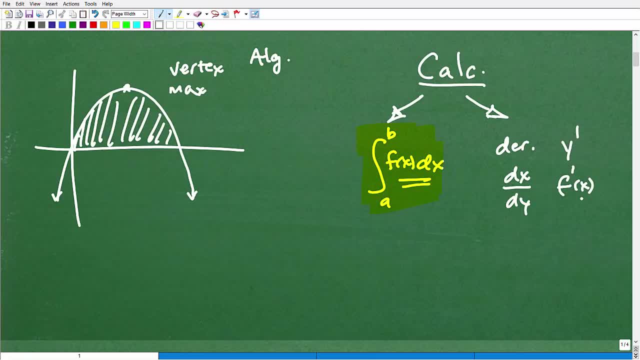 There's all kinds of ways you can. it's expressed, Okay, but we learn about the derivative. So there's like the big, huge topic in calculus is the derivative, And then we also learn about integration. Okay, in this particular problem. 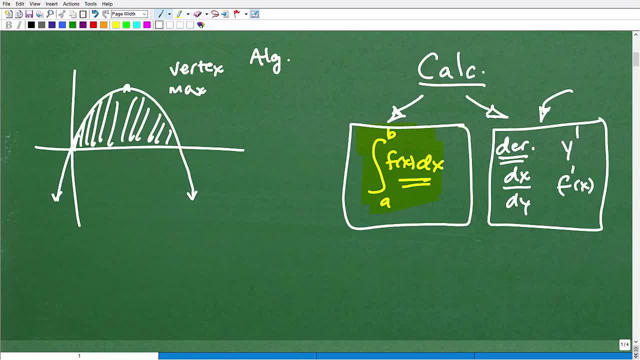 We're going to be using this concept here: the derivative, and the derivative more or less Okay, it's kind of erase all this stuff here. The derivative allows us to find the slope- Okay, the derivative has to do conceptually with the slope of something. 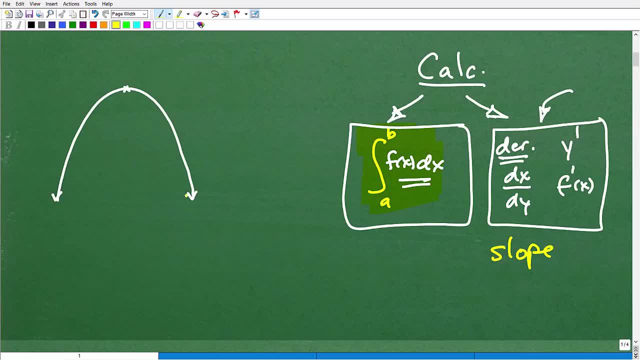 So here's my little curve, my little parabola, And along this parabola let's say at this point, right here, what's the slope of this parabola? well, it would kind of be like this line, like right here, right that. 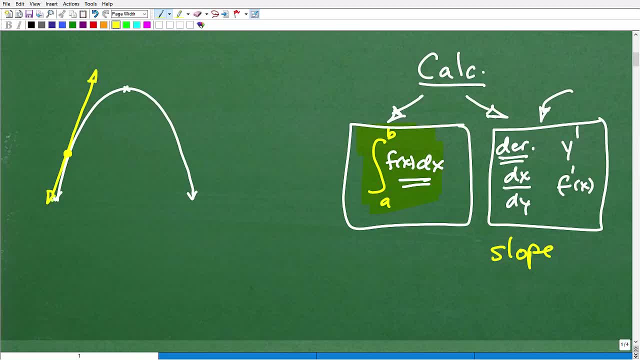 would be the slope. but what, precisely, is the slope of the parabola at this point? well, that's where we need calculus, okay, but let's just kind of follow this parabola around and this is study what the slope is looking like. how about this? 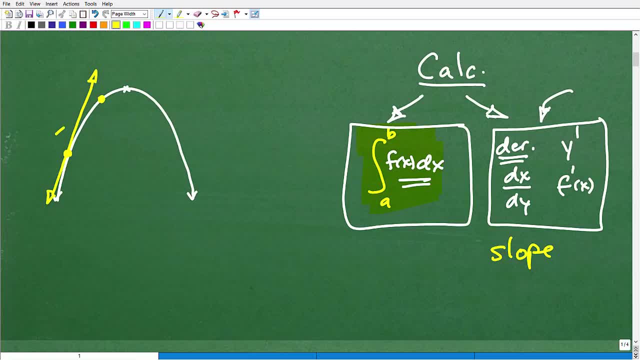 point right here. well, at that point the slope might be something like this: right, okay, so we can see the slope is changing along this parabola. how about this point right here? well, the slope is like: well, maybe like this, we kind of drew it kind of bad, something like that. now this line, okay, is what we call a tangent line. it. 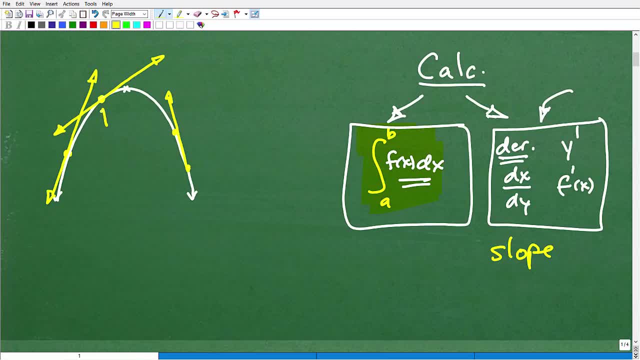 just this is one line that just touches at one single point, that parabola, at these precise points. so this, these lines are going to touch at that one point. I hear this would not be the case, but I'm just kind of sketching around here trying to make 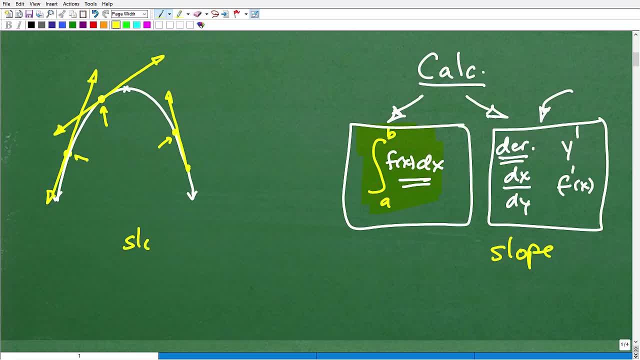 now. look, I'm writing a specific Supp히. sorry, here at the arrangediada, should be theivamente here, at the exact point now, if you don't know basic algebra, when we talk about the slope, we're talking about the angle of something, right, the steepness of something here. so the slope in this. 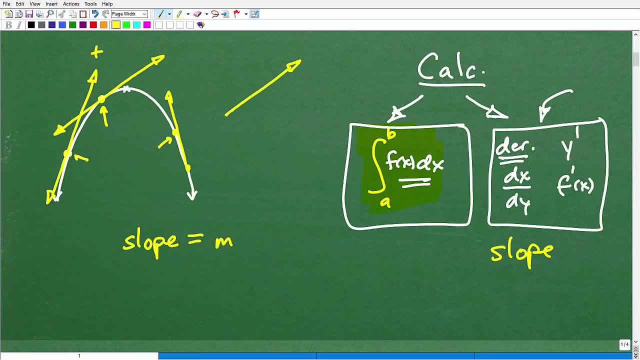 direction. we indicate that by this little variable, M is going to be positive. okay, so slopes that run like this way increase from left to right. is a positive slope, slopes that go down this way? or as a negative slope? so what, how steep is this line? okay, this is a horizontal line. you might be saying it. 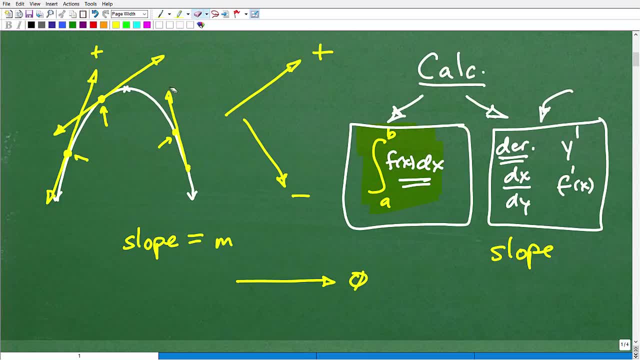 has no slope, it's zero, and you would be correct. okay, so lines that are flat, okay, or horizontal, okay, have zero slope. I'm gonna erase this here in a second. okay, so these lines, horizontal lines, have zero slope, and vertical lines- here their slope is what we call undefined. we don't really need to get into that for this. 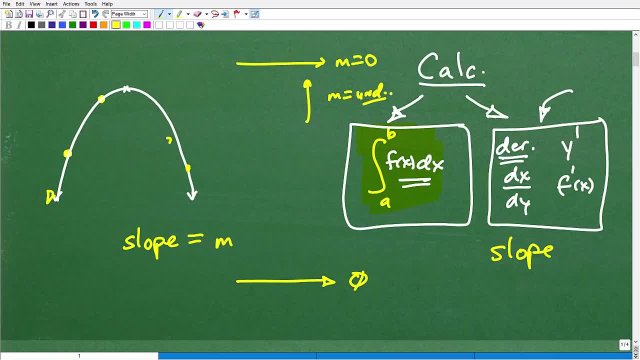 particular video. but just so you know if I'm trying to find the maximum point, just think of it as a roller coaster. this is probably good representation here. you are going up a roller coaster, you're increasing okay. so positive slope is like you're increasing on your roller coaster and then right here at the very 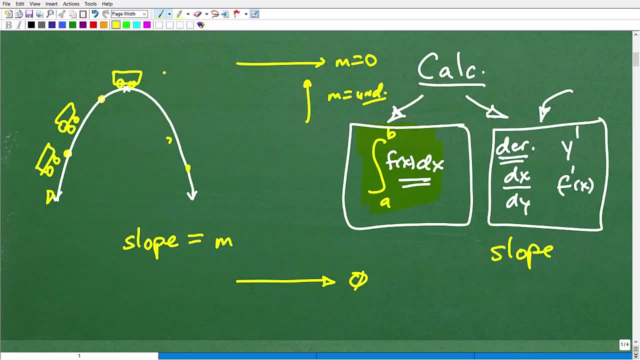 very top. you're like flat right, you're perfectly horizontal. you are like this: okay, the slope is zero. then you go down the other side. we're like this: okay, the slope is zero. then you go down the other side. we're like, okay, the slope is zero. then you go down the other side. we're like: 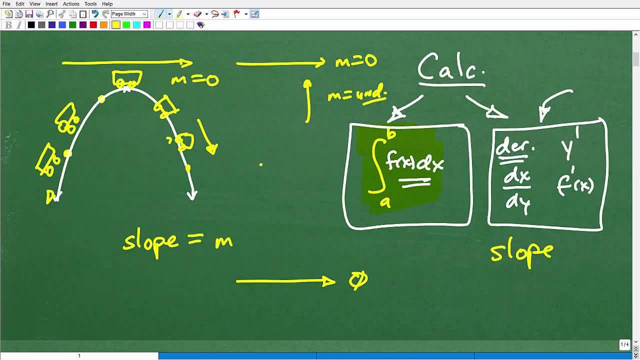 okay, and now we have negative slope. okay, so this is where the slope is negative. so this is where the slope is negative, this is where the slope is positive. and right here on the top, when everyone is just like scared, scared, scared, and then you're like, oh, you kind of go down, this is this one point, right there, okay is. 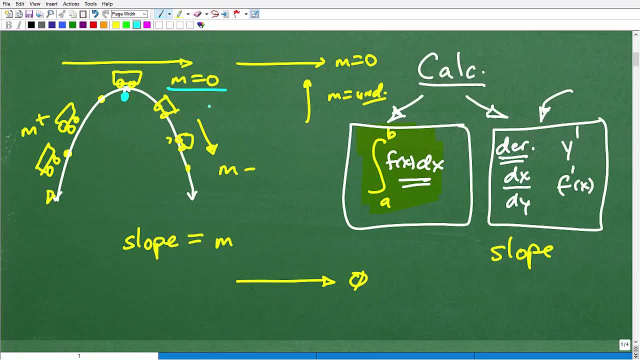 the top, okay- of the roller coaster, the top or the maximum, okay of this parabola, what we're trying to determine. now again, if you studied algebra, there's other techniques, but this is a basic, simple parabola. okay, there could be more challenging techniques that algebra can't. 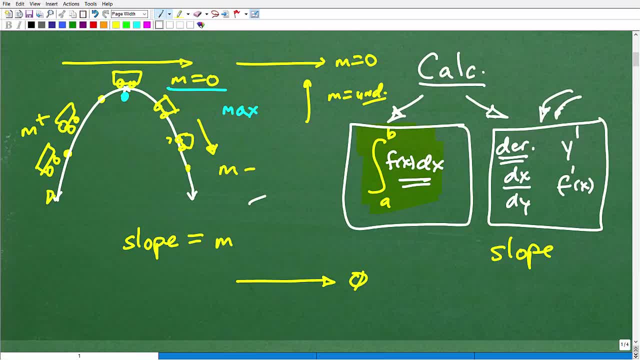 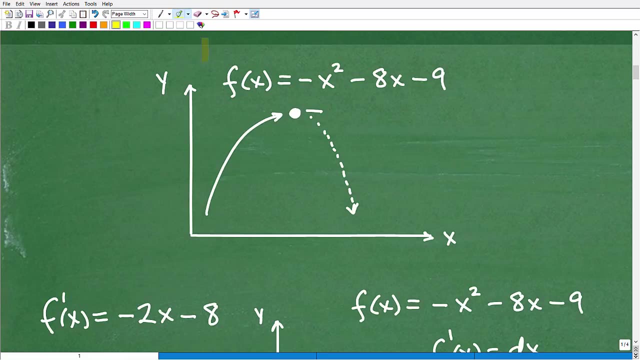 help us out and we're going to have to use our friend calculus. okay, so we're going to be using the derivative to determine the maximum of this parabola, so let's get into it now. okay, so here is our problem. okay, we want to find the maximum. now. this particular function here. okay, its graph is: 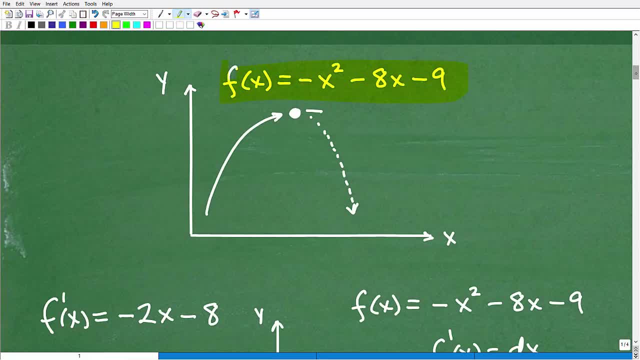 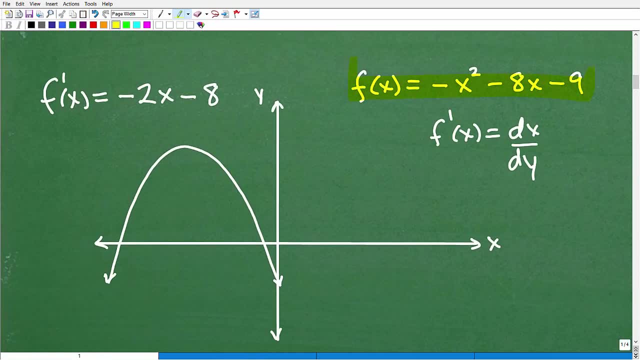 not exactly. this just kind of drew this to make it look kind of interesting. so here is this graph. this graph is really more like this on the xy plane. so here's our function, and if i was to graph this parabola, it would be like: so okay, well, again, i'm trying to find this maximum point, right. 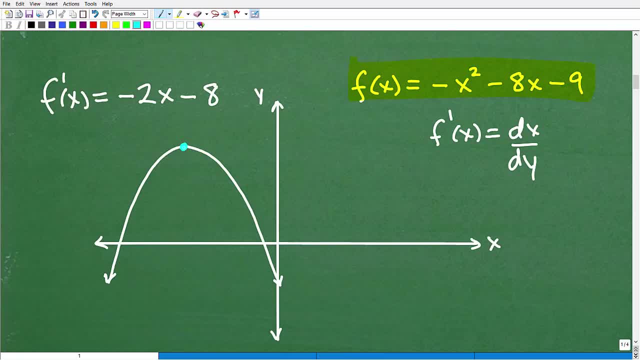 there now, that's also known as the vertex. we want to find this maximum point. okay, where does this thing max out? now, as i've indicated, we're going to use this concept here, called the derivative, and this is the notation we want to find the first derivative of. 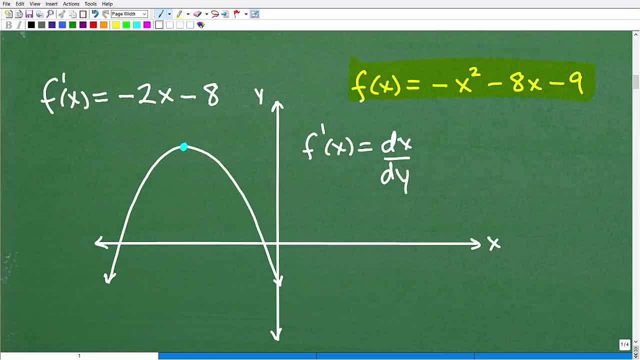 this function, okay, so this is the notation. again, dx dy. it looks like this and again, you don't need to know a lot about it, just know that we're going to find the first derivative. okay, now, let's this the function. when i find the first derivative: dx dy- okay. or f prime- okay. this, right here. this is. 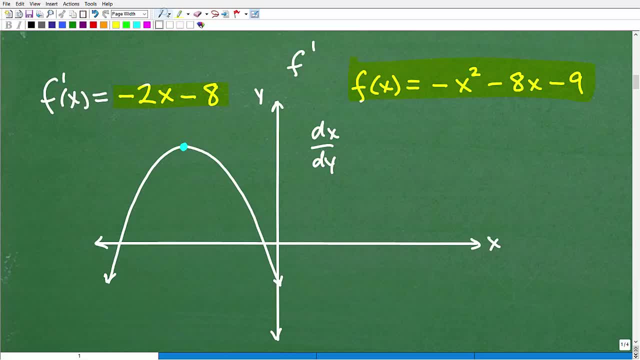 actually the first derivative i'm going to find. i'm going to show you how i got got to this. what does that mean? when i find the derivative- okay, this function right here. its graph is this parabola. there is the parabola. this thing right here is the graph of that parabola. when i find the first, 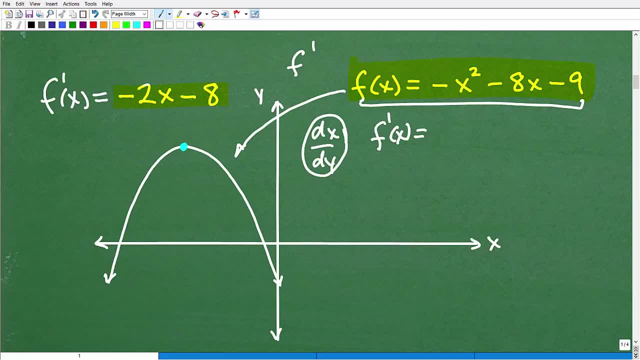 derivative. okay, these are all equivalent notations. i could write it as dx, dy, uh. or can write it like this: now notice, i said the first derivative. i could find the second derivative. that means something in more advanced mathematics, especially like physics and stuff, but i don't want to digress. 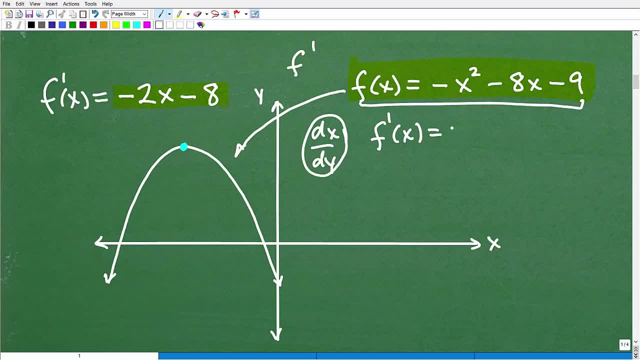 too much, because i could just get overly excited about calculus. it's such a cool topic, but anyways, here's the deal. when i find the first derivative of this function. here's the function. here's its first derivative. it's going to give me a formula for the slope, okay, so the first derivative is a. 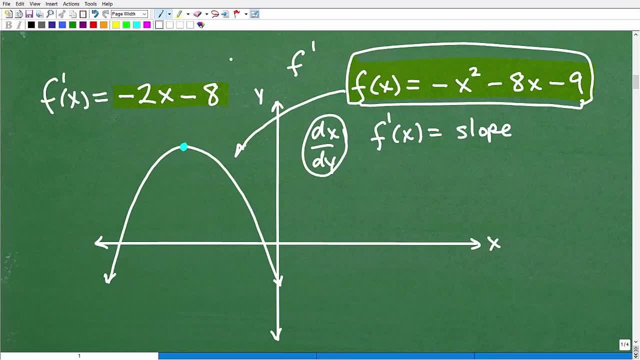 formula for the slope of anywhere along this line. this is actually the first derivative, okay, so i'm going to show you precisely what this means. so this is going to give me a derivative, a formula for the slope, or m. okay now remember, we talked about our roller coaster. m is positive here. 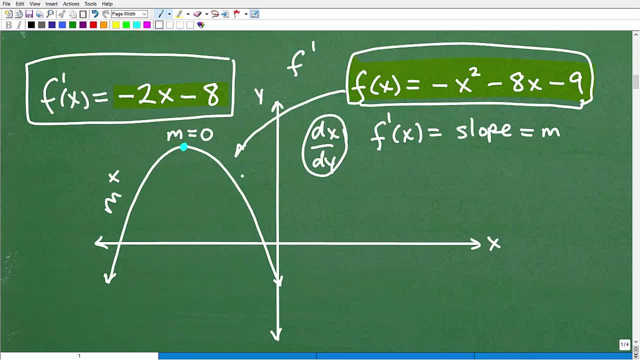 m is zero right there, okay, and then m is negative right there. so what i'm going to want to find is: where is the slope equal to zero? okay, remember, we just talked about that, because that is going to be the top of this parabola, where where the slope is zero is going to be where, uh, the maximum? okay. 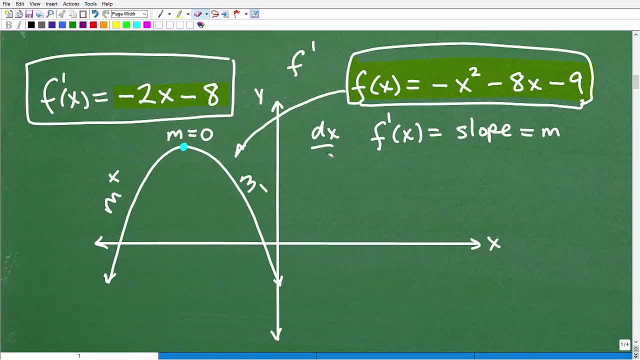 point is on this parabola. all right, so how do we find the first derivative? okay, so that's what it means. so here is how we find the first derivative. so in calculus we're given a bunch of rules. they're not that difficult, just kind of algebraic. 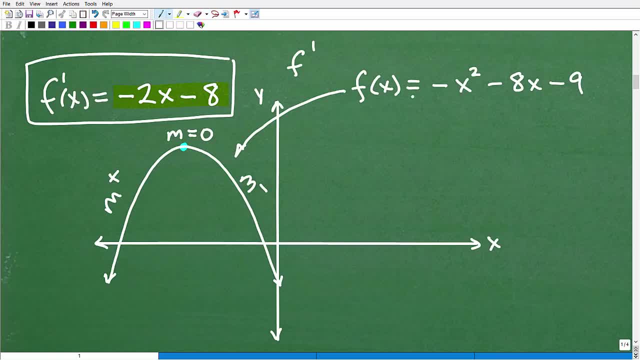 manipulations. but here is our polynomial function, our little quadratic equation, if you've taken enough algebra to understand. so here's what we're going to do. okay, to find the first derivative we're going to take. this thing is written in highest power to lowest power. we take this. 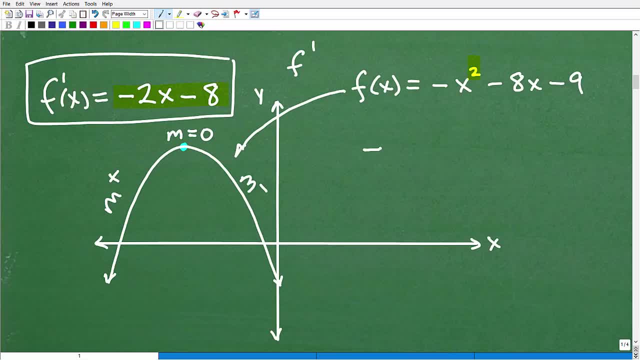 little exponent right there. okay, here let's kind of make it bigger. negative x squared. okay, so we're going to take the two. i'm going to multiply by that number, that's a negative one. okay, so it's going to be. i'm sorry, we're going to take. i'm sorry you're going to be. take the two. 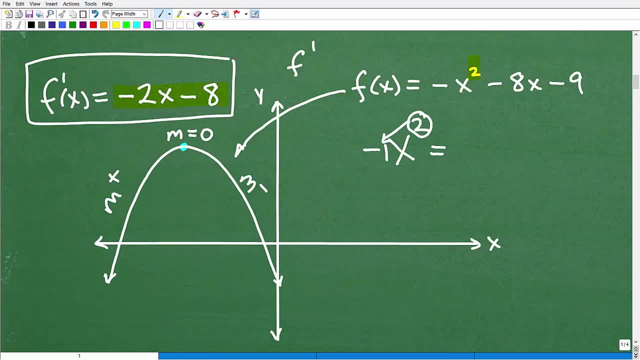 we'll multiply by that negative, uh, number, which is this one. okay, so two times negative. one is negative two, all right, so take that little two, whatever the exponent might be. if it was three, i would multiply by three. so take the two, multiply by this number that's negative one x squared. so 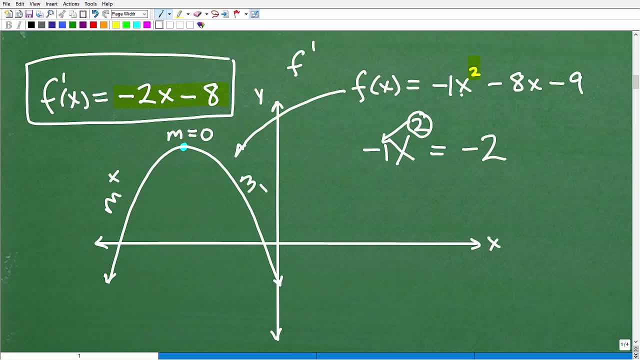 two times negative. one is negative one, so that's negative one, so that's negative one, so that's negative two. then i'm going to take that same variable x. i'm going to write it like: so, okay, and then, whatever this power is, it was two, okay, it is two. i'm going to decrease it by one, so that 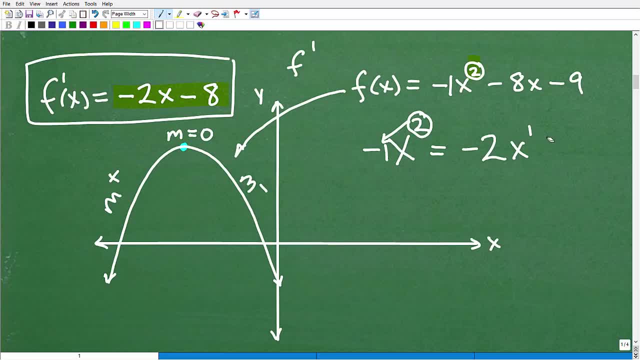 would be just to the first power one. okay, let me do that again. all right, so we can understand this rule. to take: have a function, a polynomial function, to be able to find the first derivative. it's not that difficult. so we have negative x squared. okay, i take the two, multiply by this number, which is just a negative one. two times negative one is: 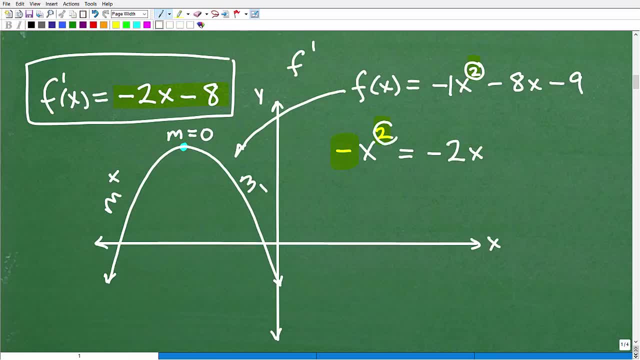 negative. two, it's the variable x. now, whatever this is, i'm going to drop it down by one, so that's two to the first, or just two? okay, i could write it just like that, and that is step one. okay, now i'm going to do the same thing over here, all right. so what's the power of this? it's one, okay, so it's. 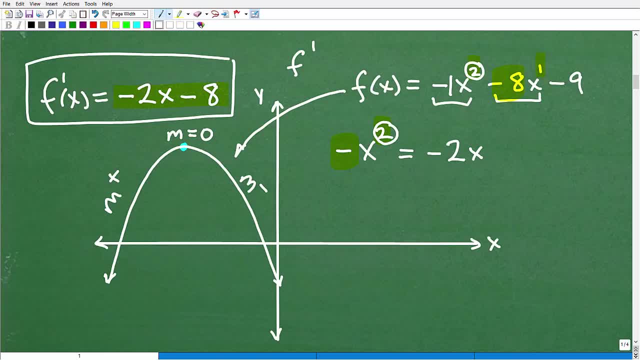 going to be one times negative one, and i'm going to do the same thing over here. all right, so it's negative eight. is what negative? eight times x two, this is one. i'm going to drop it down by one, so that's x to the zero. anything to the zero, power is one. anything to the zero, power is one. 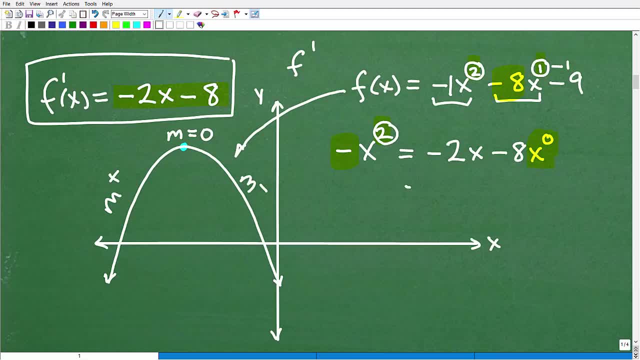 so that's really negative eight times one. so my first derivative is negative two x minus eight, because it's negative eight times one. this is really just one. and then you're taking a derivative of a number. it's just zero, it goes away, okay. so this here is our first. 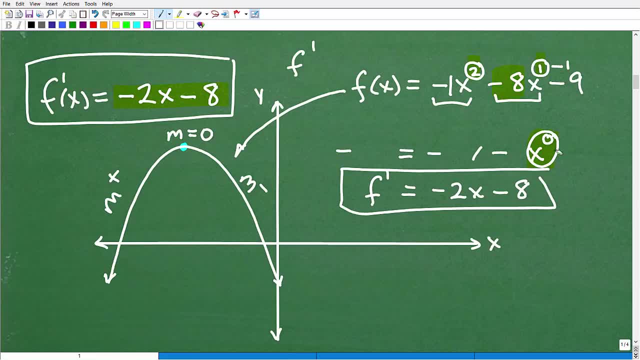 derivative. again, i'm using different notation here. it's the function x, okay, f of x. so all equivalent notation. what we just found is the first derivative of this function, f. so it can be written as dx, dy, very, very common. okay, or we write this little apostrophe. that's the first. 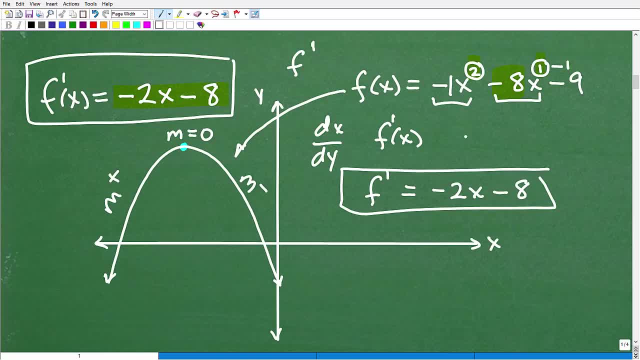 derivative of the function f. or we can write this little apostrophe: that's the first derivative of this function, f. or this function's name is f. i can write it like this: okay, all equivalent f prime. we would call this: okay, f prime, first derivative of this function. again, this is a lovely formula. 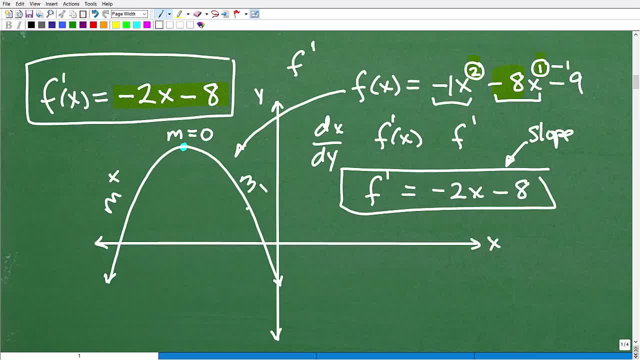 for the slope. okay, it's going to tell me where the slope is at now i'm interested in where is the slope equal to zero? okay, remember? okay, just a quick review. the slope is positive in this direction. its slope is negative in this direction, but at this one precise point. 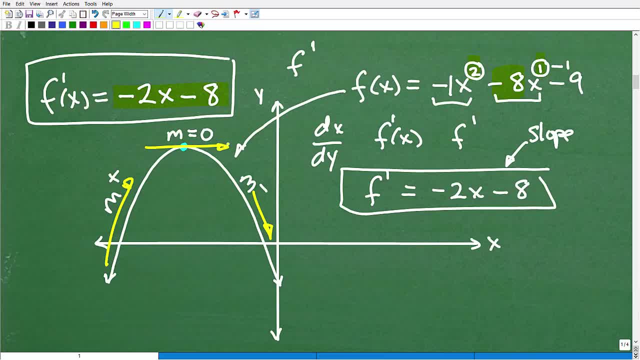 at the top of the roller coaster, the slope is zero. all right, so let's find that point now. okay, erase all of this, okay. so here is my formula for my slope. i know my slope along this function, along this parabola, is equal to negative two x minus eight. so i'm gonna, i want to say to myself: 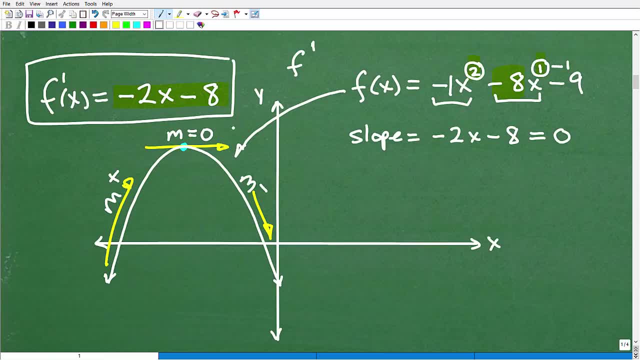 okay, mr slope, where are you equal to zero? because that's where i'm interested in knowing. okay, where the slope is equal to zero. so i'm going to set the slope, the formula uh, or the equation here for the slope equal to zero and i'm going to solve that equation. so negative two x minus eight equals. 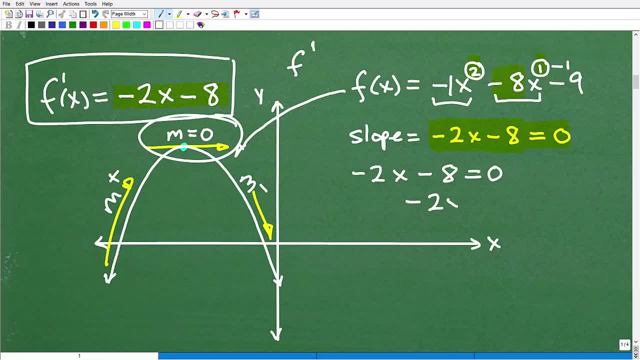 zero. i'm going to move the eight over to the other side of the equation, that's negative two. x is equal to eight and i'm divide both sides equation by negative two, so x is equal to negative four. okay, so right here, um one, two, three, four, negative four, along where x is negative four. at this point that is the maximum. 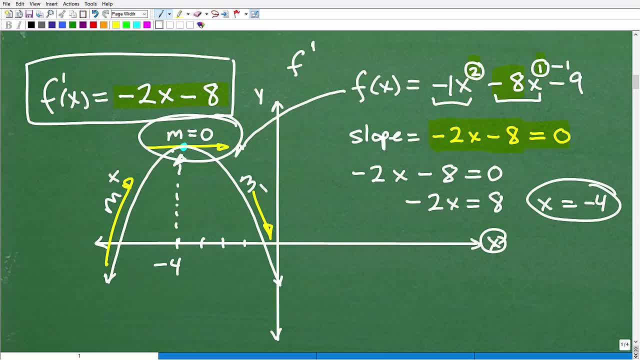 along the x-axis of where that's at, and if i wanted to know this exact coordinate, i would just plug in negative four into my original function, and i actually just did that right here. okay, let's plug in negative four into our original function to find out what the y. 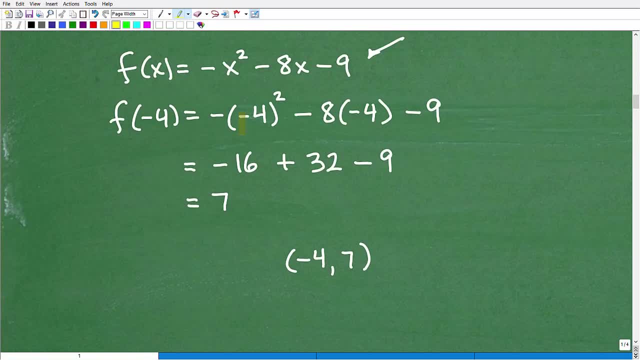 coordinate is. and when i do that, whoops. you can see here i'm plugging in very precisely negative four. here i do all the math. and f of negative four for this function is seven. so the top of that parabola- okay, right there, okay- is located at one, two, three. 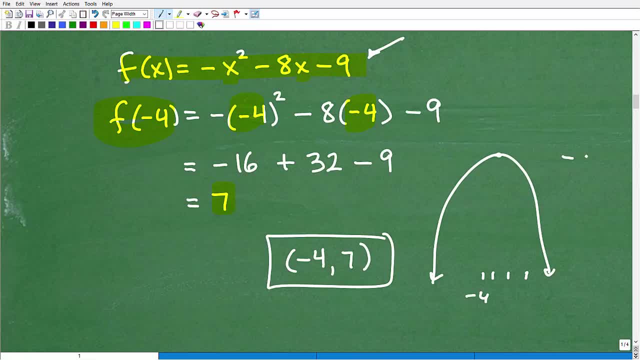 four. negative four. seven. okay, seven, this way, all right, not negative seven, but seven in this direction, right there, so that vertex, that maximum point for this parabola, occurs at negative seven. now, uh, this is an illustration of using the first derivative okay, of a function, all right to solve. 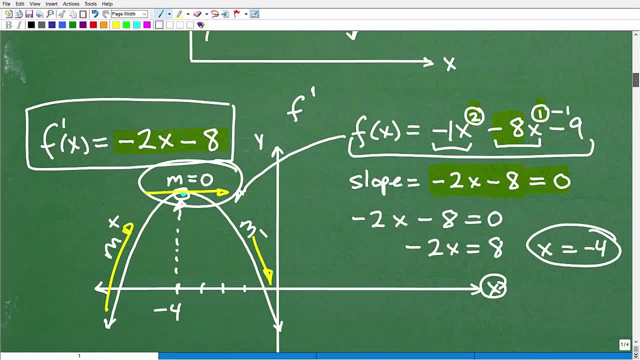 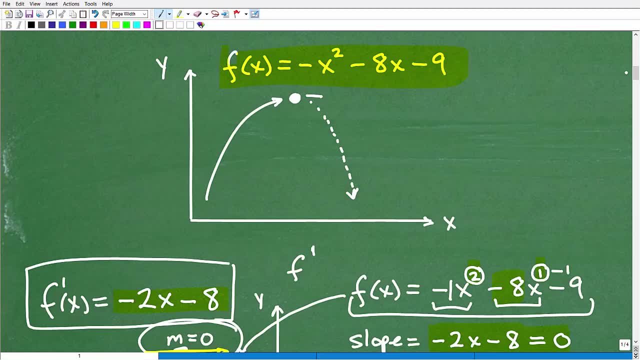 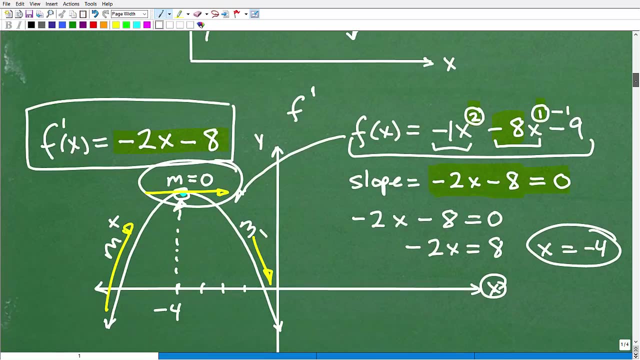 a problem. now there is another way, more direct approach. we can use algebra, but this is a an easy problem. okay, uh, algebra can, you know, help us with the easy problem. but then there's a lot of other things that calculus, just you know, cannot help us with. all right, we you know, but i, you know, chose. 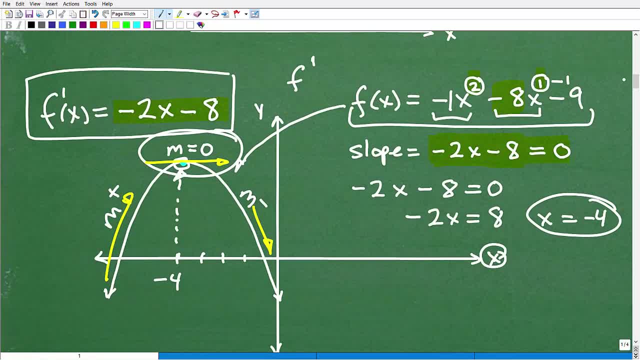 this because this is our first calculus problem together. i wanted to say that we're going to use this to make sense for uh to you and hopefully, even if you didn't get all the algebraic manipulations and i think, um, hopefully you can understand the concept of the roller coaster stuff. 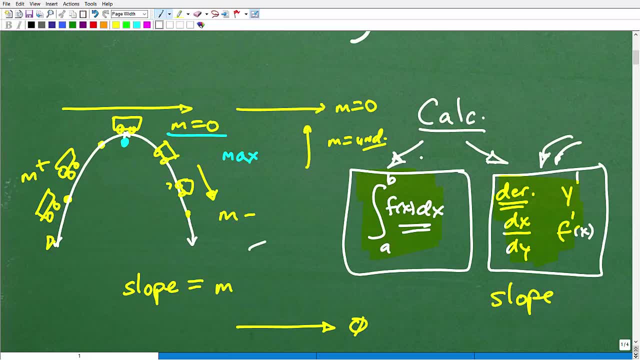 here and get an appreciation for the basic, main basic concepts of calculus, integration and- uh, the derivative. all right, now again, you know i'm oversimplifying a lot of things and if you have, you know, a pretty advanced math background you might be saying, oh, you missed that, you missed. 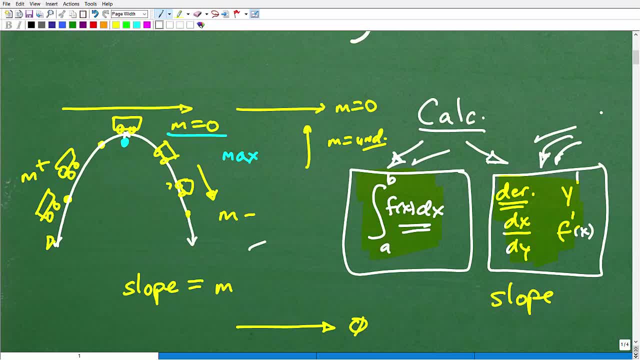 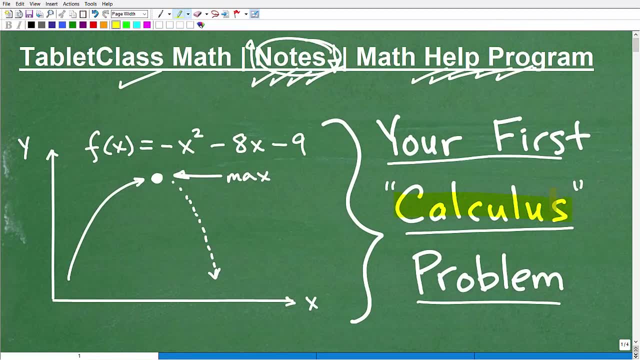 this. yes, listen, i get that right. i'm not trying to teach a full calculus course here. that's just the point of this video. the point is to teach you a little something about the subject of calculus so you can appreciate it and maybe even get motivated enough, excited about it, enough to be 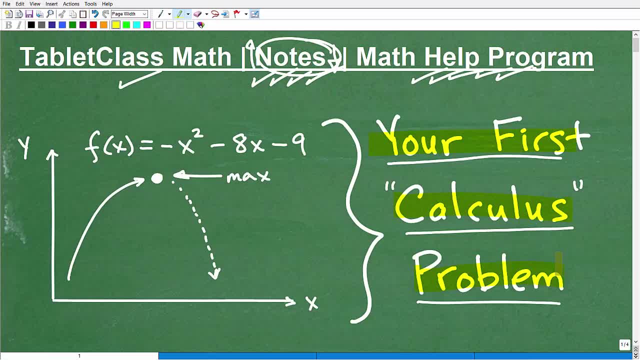 like: you know what i want to learn this uh subject? okay, it's definitely uh a great goal. you might be like: yeah well, you're a math teacher, you love math. of course you're going to like want everyone to know calculus. like, yeah well, it is a math teacher, you're going to want everyone to know calculus. 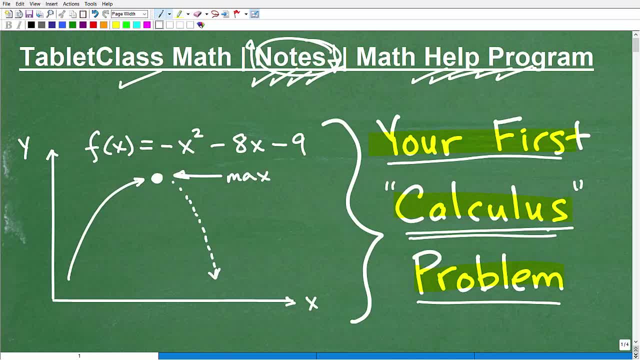 because people just don't realize, okay, without calculus, um, all our modern day technology would just fall apart. right, calculus has solved so many problems, uh, technical problems. we just would not be here without calculus. we wouldn't have our cell phones, we wouldn't have, uh, airplanes, yada, yada, yada. 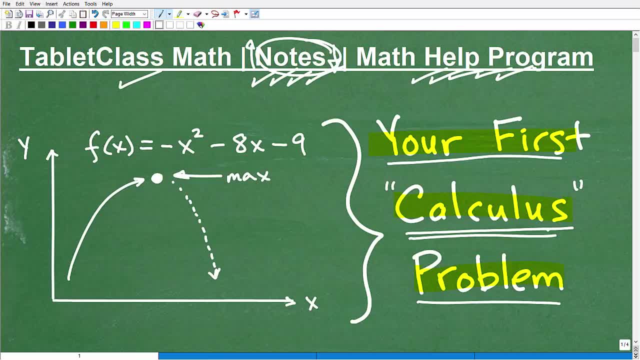 okay, anyways, i don't want to start preaching here about calculus, importance of it, but it's just a fascinating, uh, mathematic subject and it does take. you know it is a serious subject. you do have to really build up your math skill sets, uh, to be prepared to. 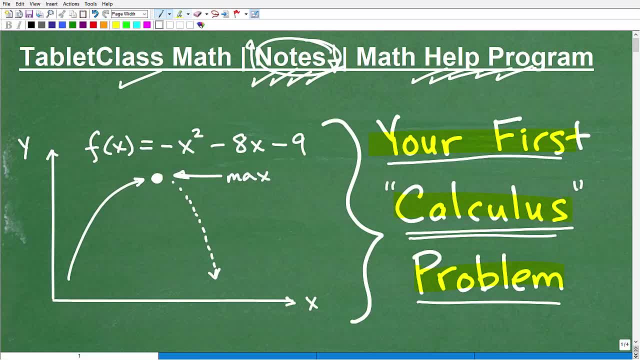 actually take it in a formal way, but i think that would be a noble goal for sure. well, if you found this video entertaining, interesting in some way or helpful, uh, definitely appreciate you smashing that like button. that helped me out. and, uh, if you're new to my youtube channel, hopefully you'll.